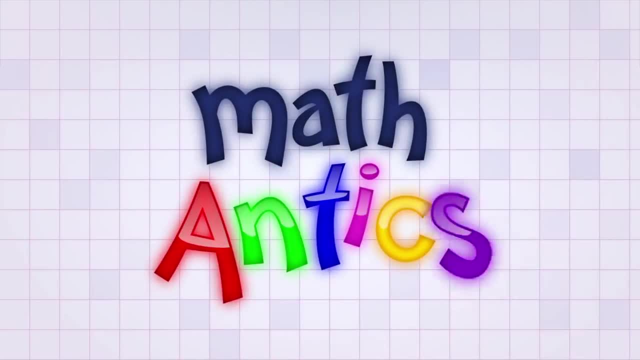 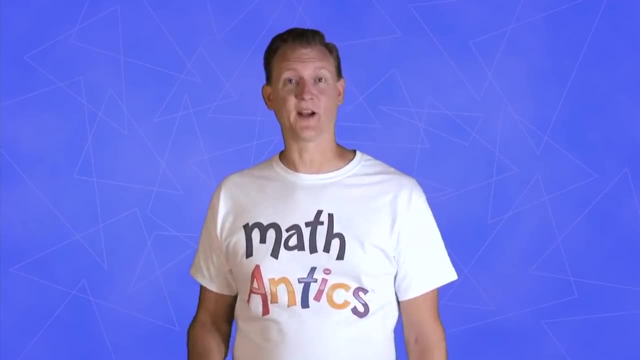 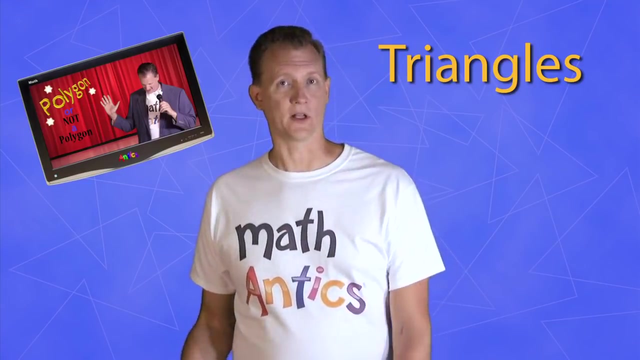 Hi, welcome to Math Antics. In this geometry lesson we're going to learn all about triangles. You may remember from the lesson about polygons that triangles are special polygons that always have three sides and three angles, And that's what the word triangle means. 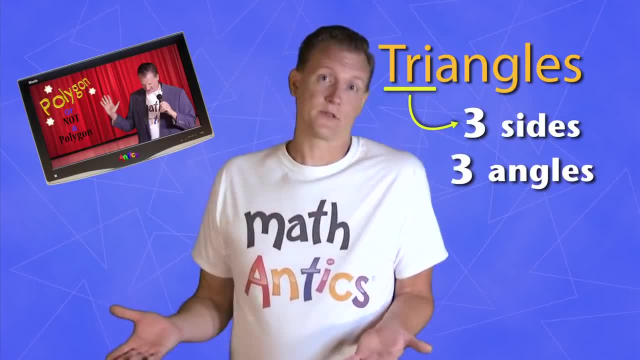 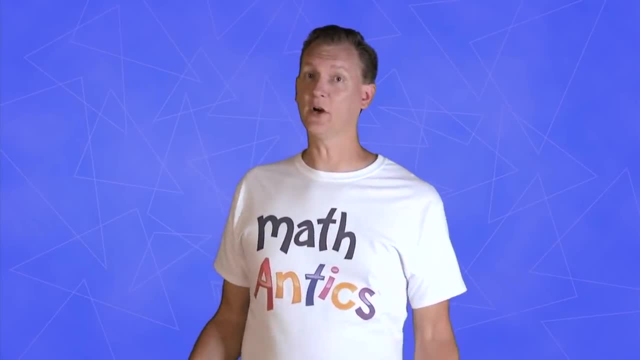 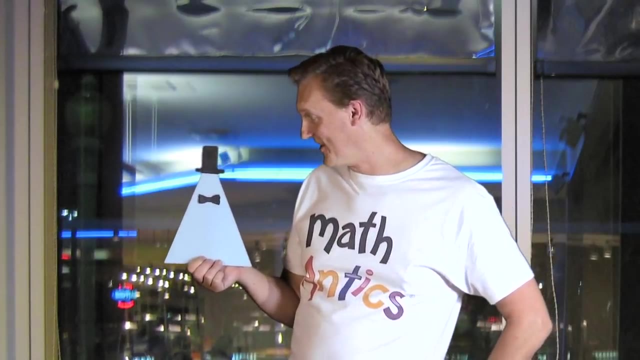 Tri means three, and angles means angles. Okay, that's easy enough: Three sides, three angles. But what else is there to know about triangles? Well, for starters, we're going to learn how to classify triangles. Oooh, such a classy triangle. 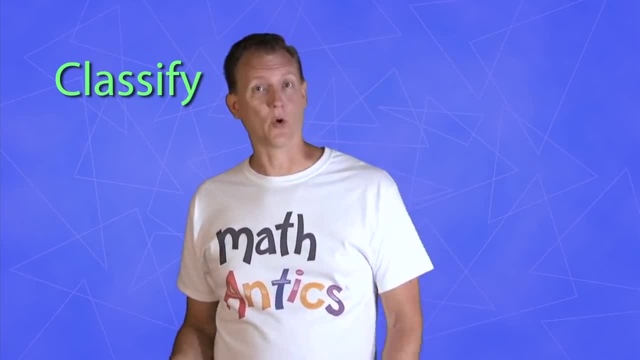 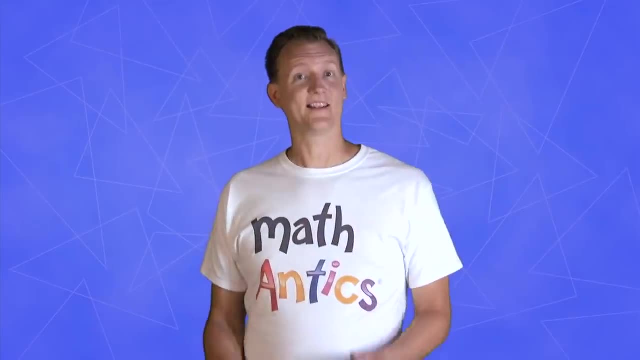 But seriously, there's two different ways to classify or organize triangles: They can be classified by their sides and they can be classified by their angles. Let's start by classifying triangles by their angles, since we've already learned a lot about angles in the previous videos. 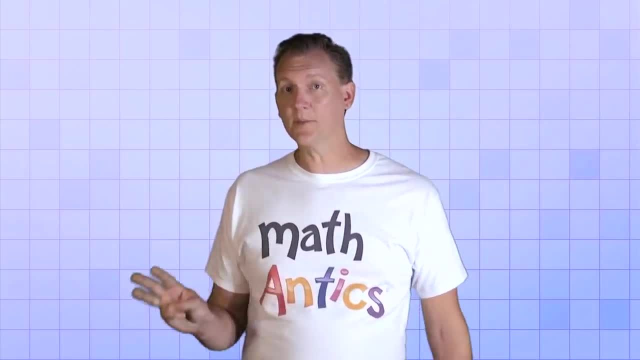 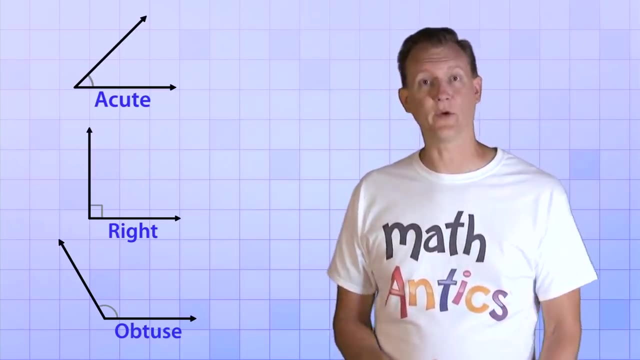 You may remember from our first video about angles that there's three types of angles. There's right angles, acute angles and obtuse angles. Well, watch what happens if we use a third line in each of these angles to form closed shapes. 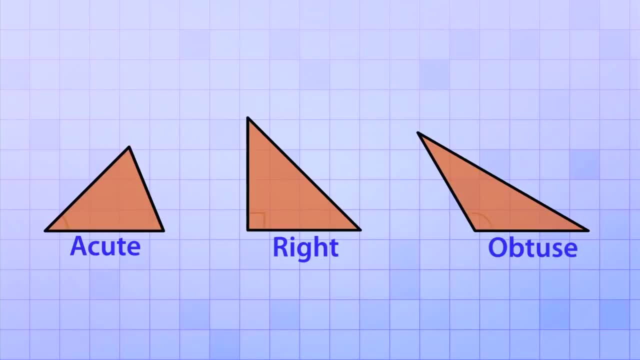 Aha, Triangles. And can you guess what these three different kinds of triangles are called? Yep, the one made from the right angle is called a right triangle, The one made from the acute angle is called an acute triangle And the one made from the obtuse angle is called an obtuse triangle. 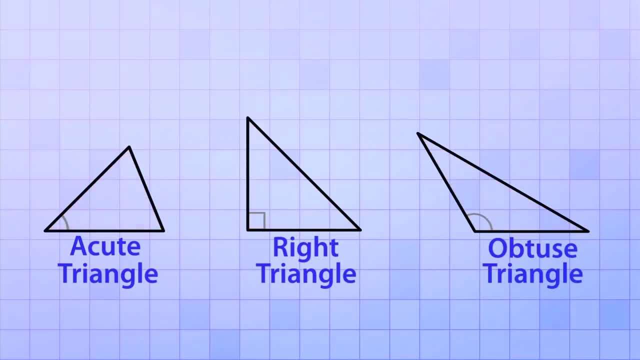 So that's simple enough. But notice that for each of our three triangles, the new angles that were formed when we closed the shapes are all acute angles. So triangles always have at least two acute angles, And it's the other angle that determines what type it is. 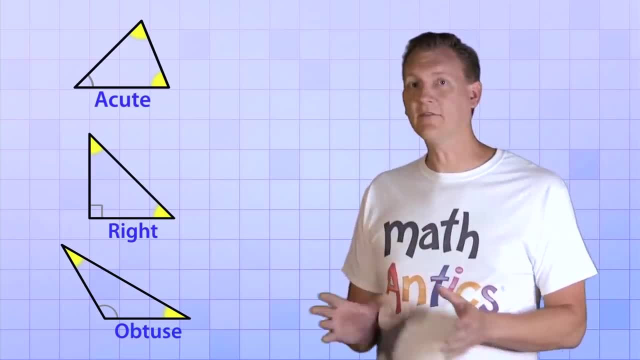 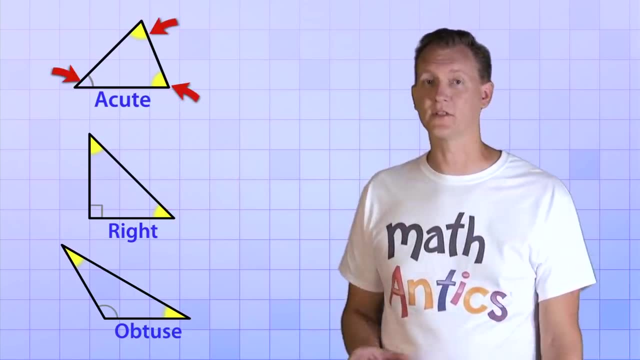 That's important to know so you don't get tricked For any given triangle: just because you see one acute angle, that doesn't mean it's an acute triangle. You have to look at all the angles to tell if it's an acute triangle. 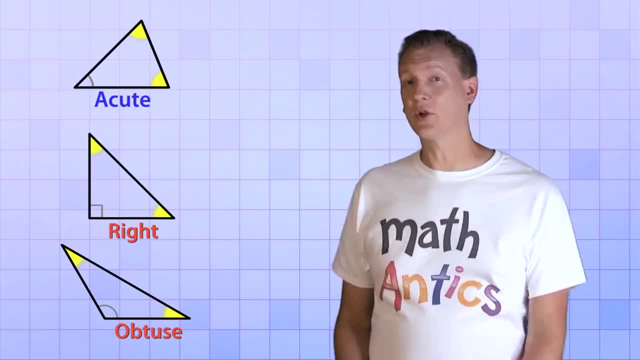 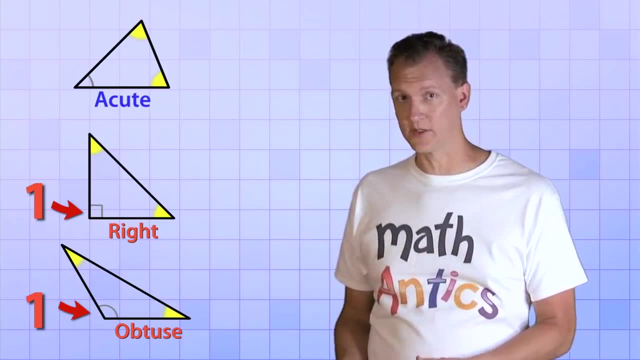 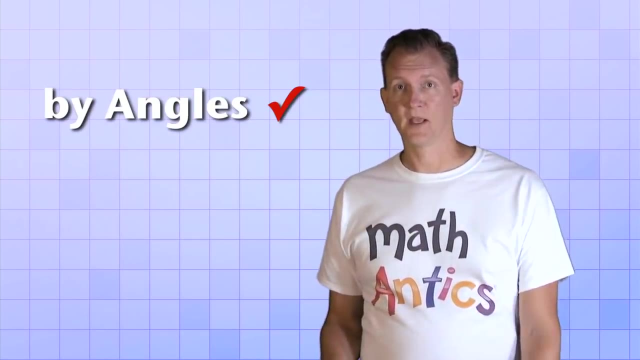 The situation's easier with right and obtuse triangles, because you can only have one right or obtuse angle per triangle. So as soon as you spot one of those kinds of angles, you know what type of triangle you have. All right, then. classifying triangles by angles is pretty simple. but we can also classify 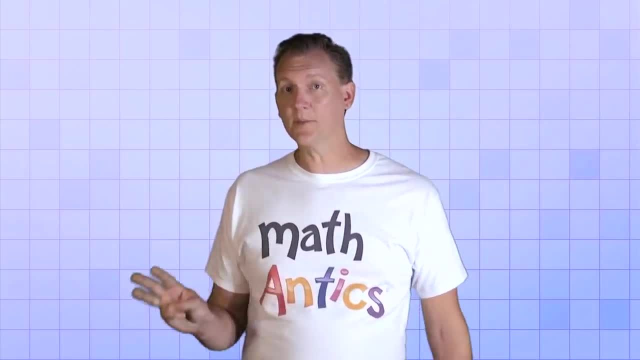 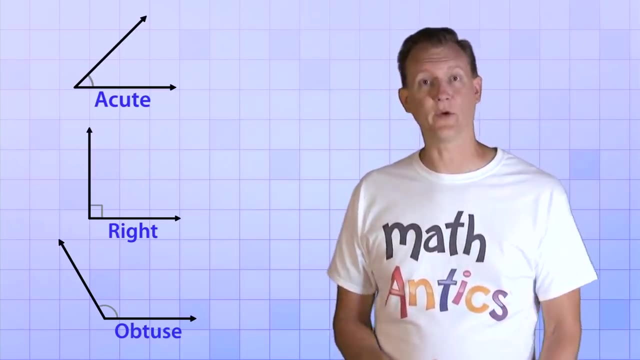 You may remember from our first video about angles that there's three types of angles. There's right angles, acute angles and obtuse angles. Well, watch what happens if we use a third line in each of these angles to form closed shapes. 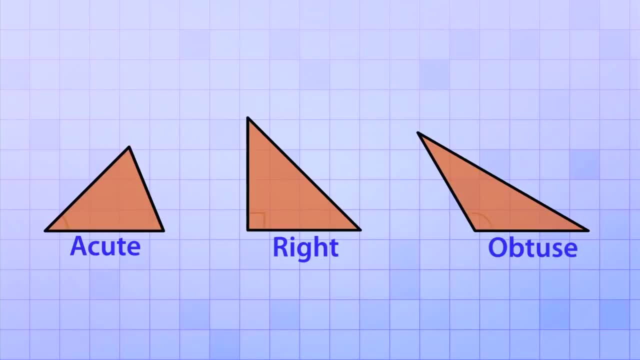 Aha, Triangles. And can you guess what these three different kinds of triangles are called? Yep, the one made from the right angle is called a right triangle, The one made from the acute angle is called an acute triangle And the one made from the obtuse angle is called an obtuse triangle. 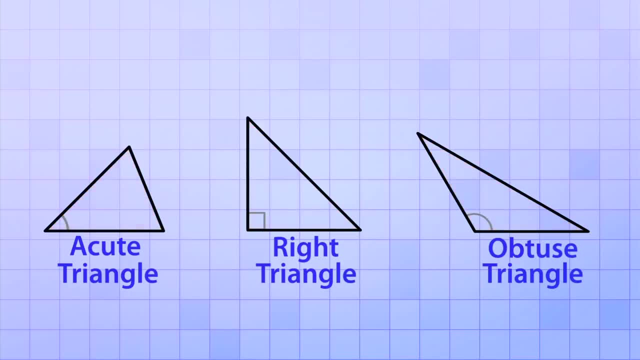 So that's simple enough. But notice that for each of our three triangles, the new angles that were formed when we closed the shapes are all acute angles. So triangles always have at least two acute angles, And it's the other angle that determines what type it is. 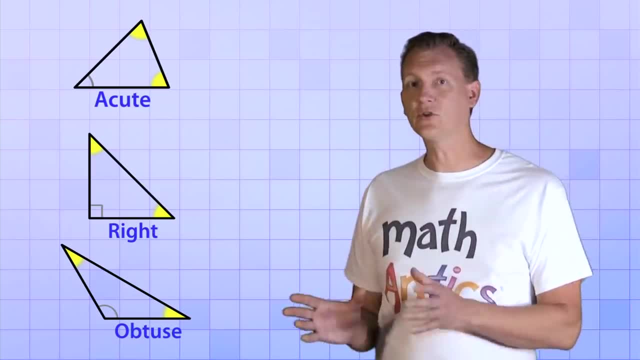 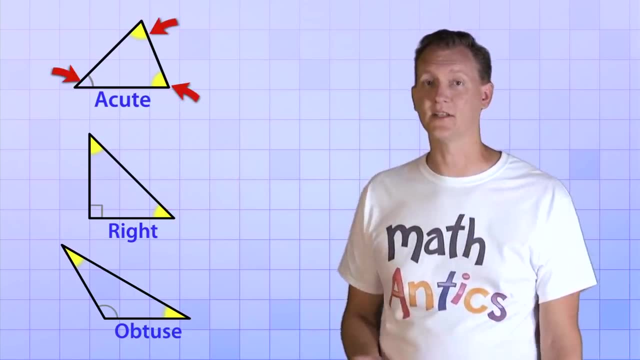 That's important to know so you don't get tricked For any given triangle: just because you see one acute angle, that doesn't mean it's an acute triangle. You have to look at all the angles to tell if it's an acute triangle. 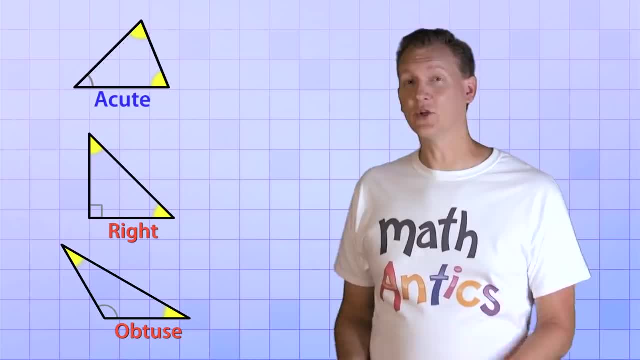 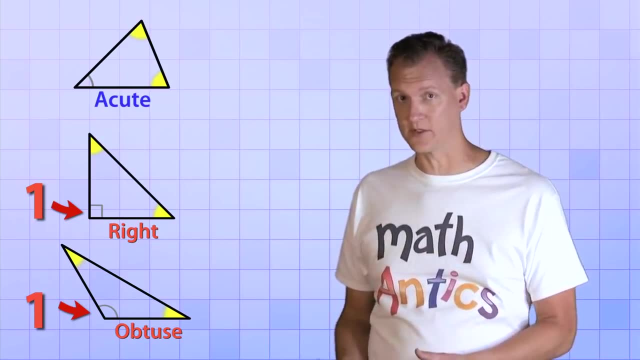 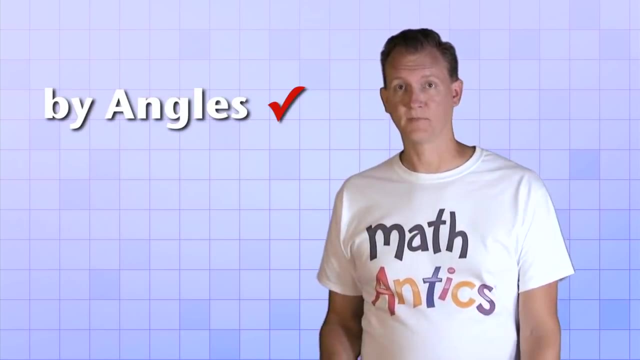 The situation's easier with right and obtuse triangles, because you can only have one right or obtuse angle per triangle. So as soon as you spot one of those kinds of angles, you know what type of triangle you have. Alright, then classifying triangles by angles is pretty simple. 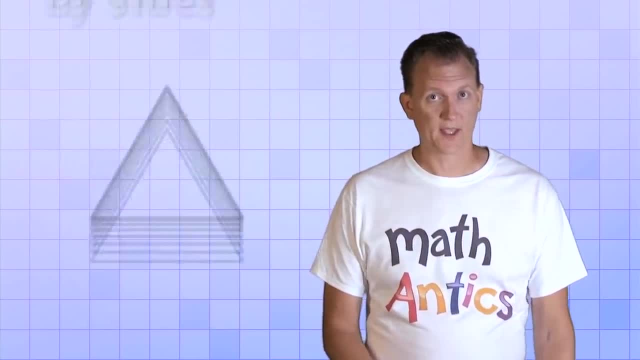 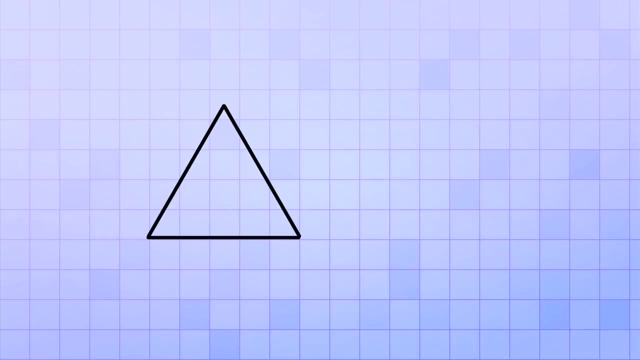 But we can also classify triangles by angles. We can also classify triangles by their sides. If we pay close attention to the length of each side of a triangle, we can see that there's three possibilities. First of all, if all three sides of a triangle are exactly the same length, then we call it an equilateral triangle. 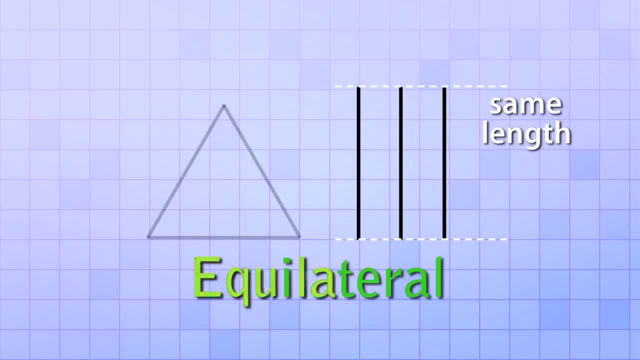 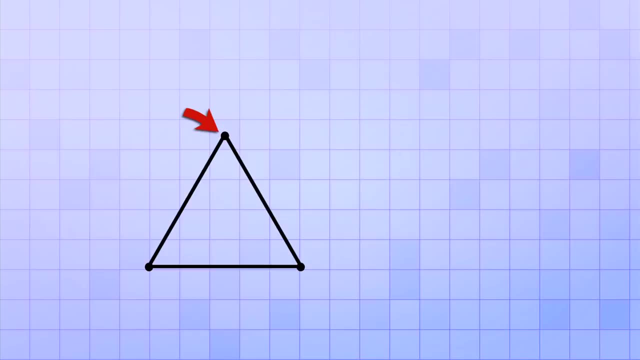 It's kind of a long word but it's easy to remember because it sounds like it has the word equal in it. To see the second possibility, let's take the top vertice of our equilateral triangle and move it up like this: 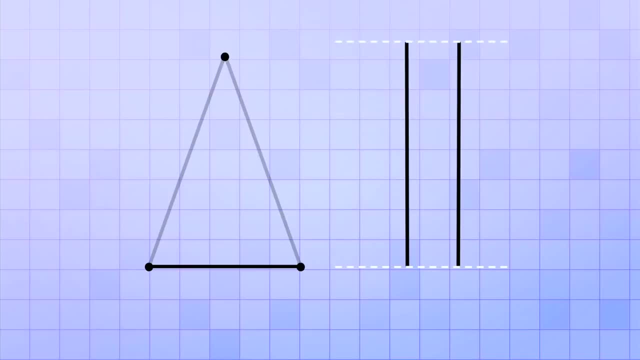 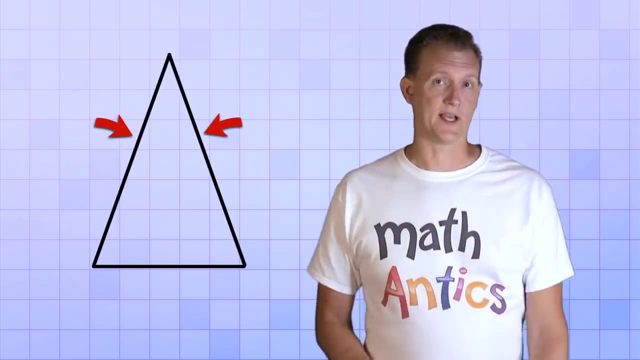 See what happened. Two of the triangle's sides got stretched by the same amount, But the bottom side remained the same. Now we have a triangle that has only two equal sides, And that's called an isosceles triangle. That's a long word too. 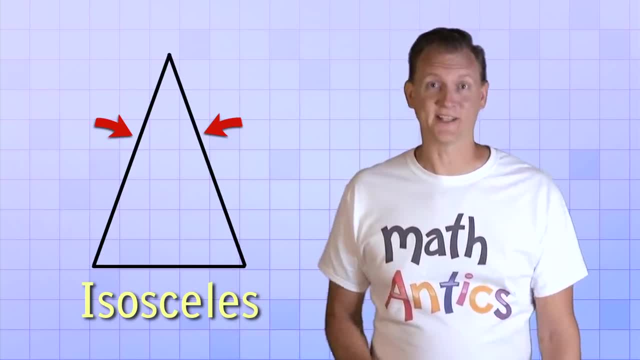 The best way to remember that is to look at an isosceles triangle and say its name 20x as fast as you can: Isosceles, isosceles, isosceles, isosceles, isosceles…. 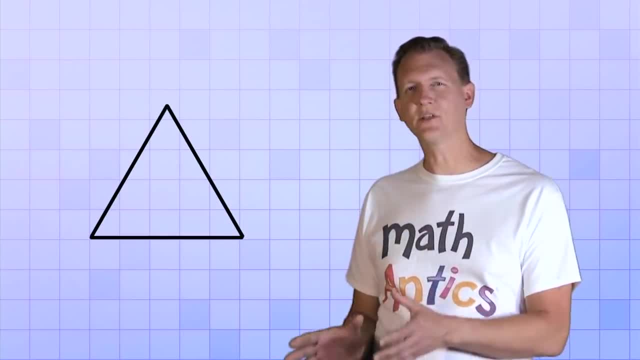 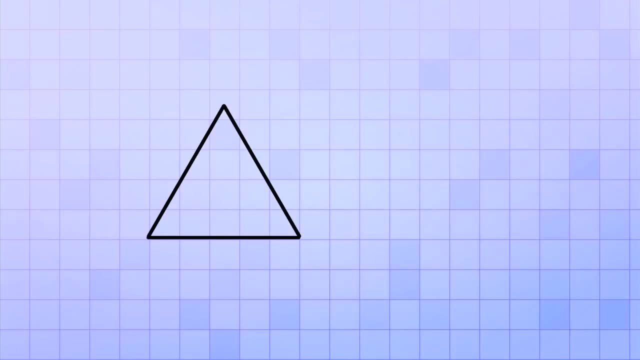 triangles by their sides. If we pay close attention to the length of each side of a triangle, we can see that there's three possibilities. First of all, if all three sides of a triangle are exactly the same length, then we call it an equilateral triangle. 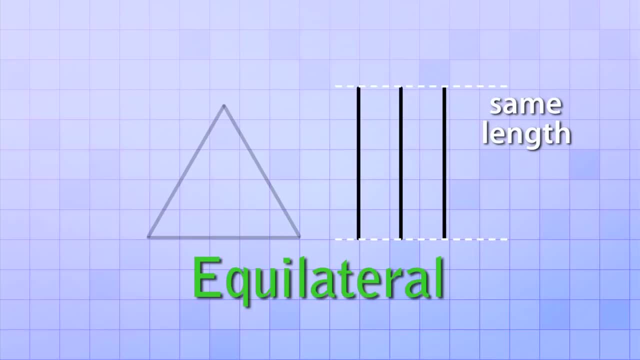 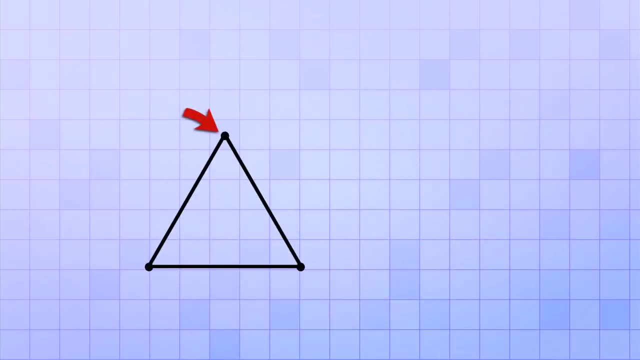 It's kind of a long word but it's easy to remember because it sounds like it has the word equal in it. To see the second possibility, let's take the top vertice of our equilateral triangle and move it up like this: 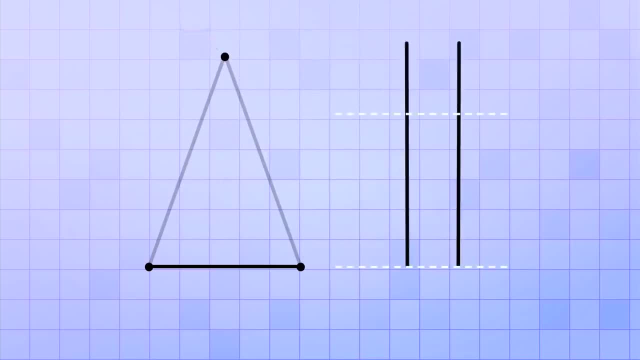 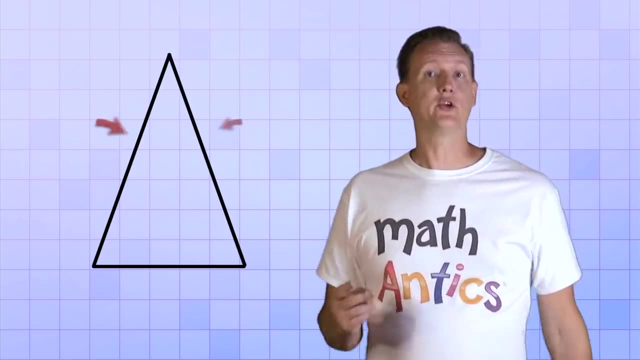 See what happened. Two of the triangle's sides got stretched by the same amount, but the bottom side remained the same. Now we have a triangle that has only two equal sides, and that's called an isosceles triangle. That's a long word too. 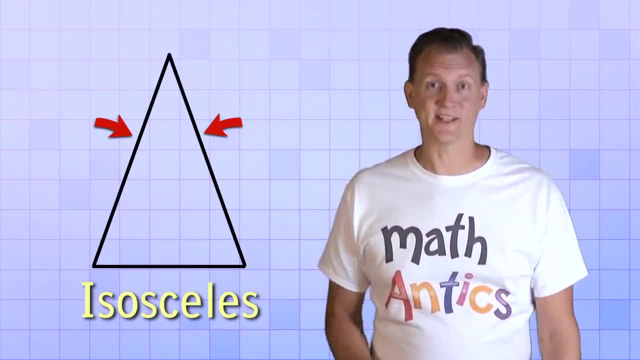 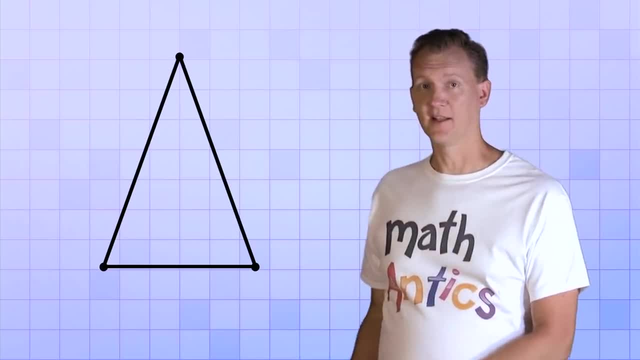 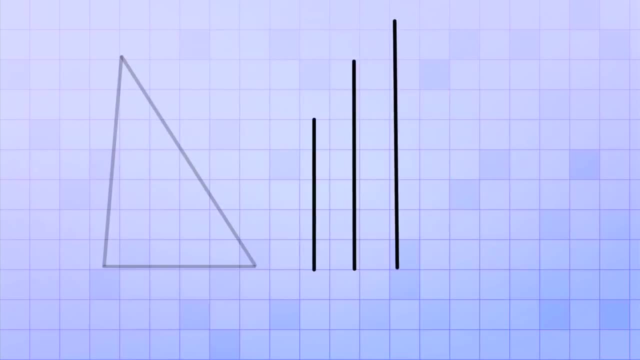 isosceles, isosceles. And finally, to see the third possibility, let's move that same top vertice This time to the left. Now all the sides are different lengths. This type of triangle is called a scalene triangle. 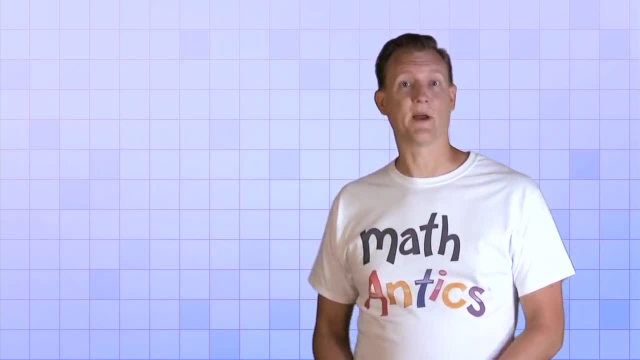 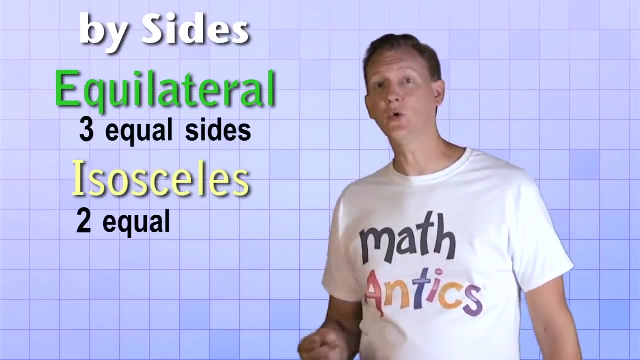 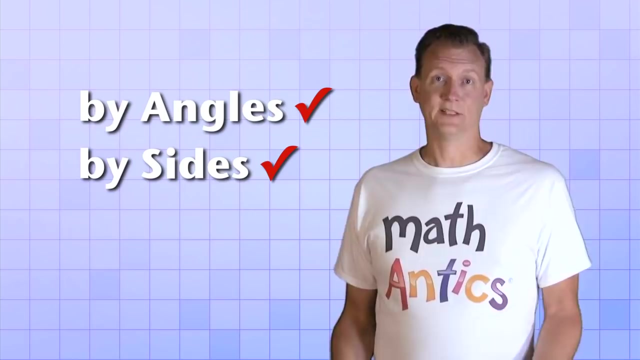 So those are the three possibilities when classifying triangles by their sides. Equilateral triangles have three equal sides, isosceles triangles have only two equal sides, and scalene triangles have no equal sides. That way was pretty easy too. The hardest part is just remembering the names. 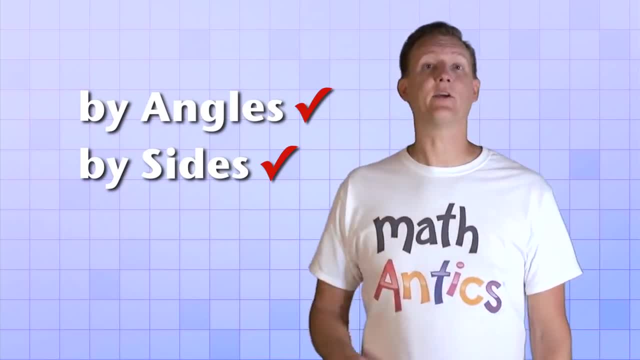 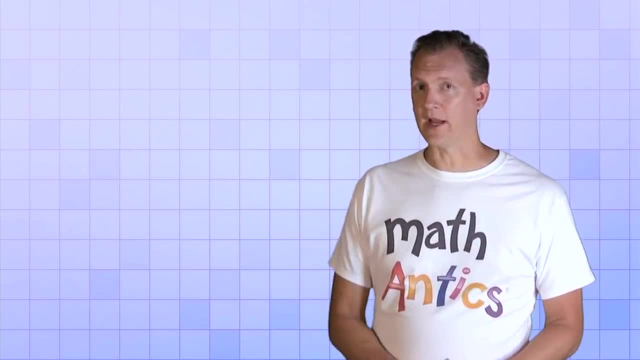 And now that you know both ways to classify triangles, let's see how you can use them together. Yep, you can use them both at the same time. If you classify triangles both by their angles and by their sides, it turns out that there: 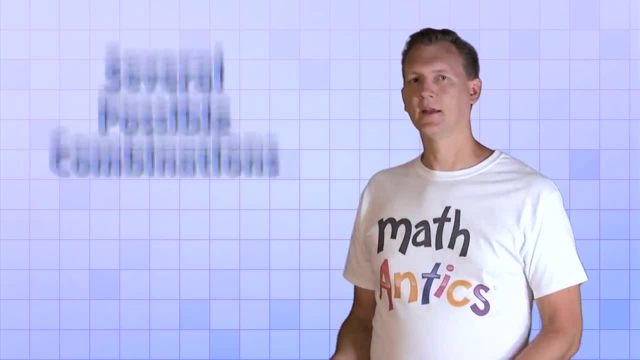 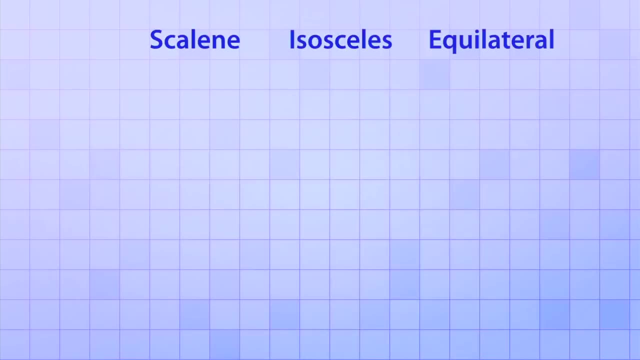 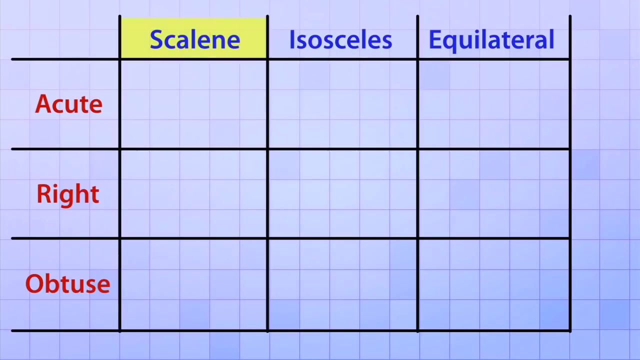 are several possible combinations. To see what I mean, let's list the three classifications by sides- scalene, isosceles and equilateral- and the three classifications by angle: right, acute and obtuse. A scalene triangle can also be a right triangle, like this one. 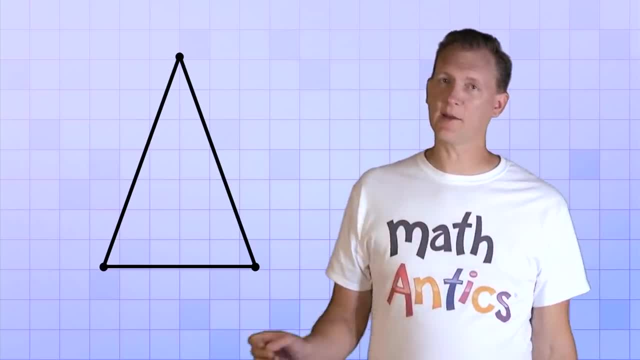 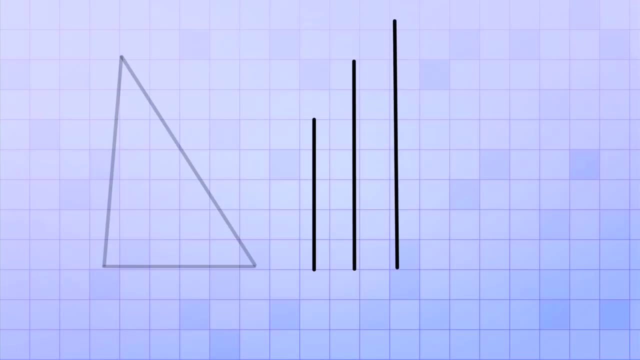 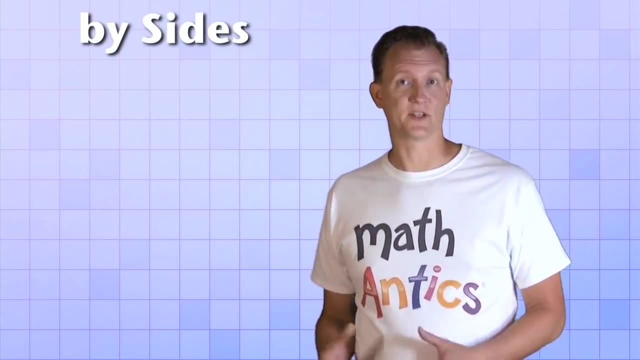 And finally, to see the third possibility, let's move that same top vertice again, but this time to the left. Now all the sides are different lengths. This type of triangle is called a scalene triangle. So those are the three possibilities when classifying triangles by their sides. 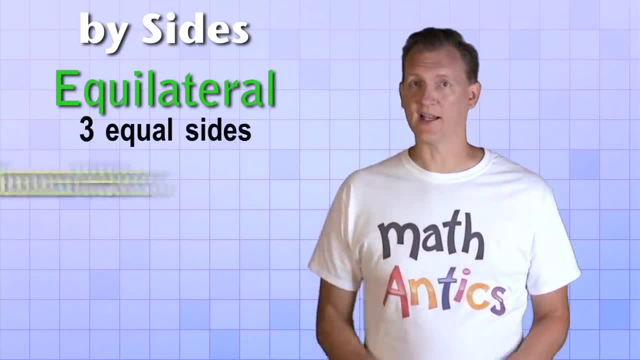 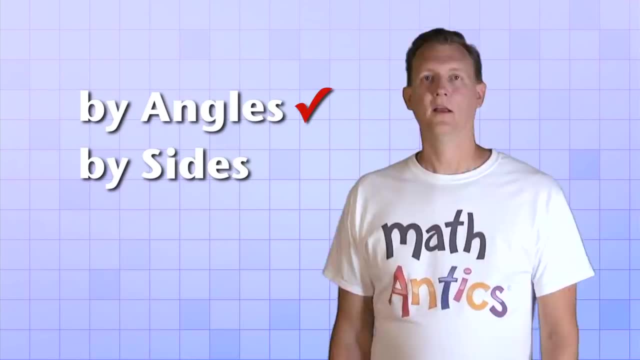 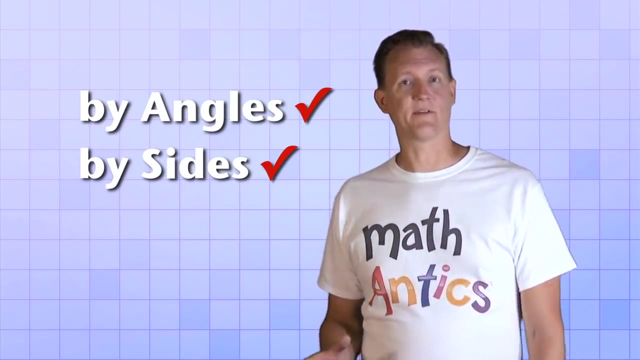 Equilateral triangles have three equal sides, Isosceles triangles have only two equal sides And scalene triangles have no equal sides. That way was pretty easy too. The hardest part is just remembering the names, And now that you know both ways to classify triangles. 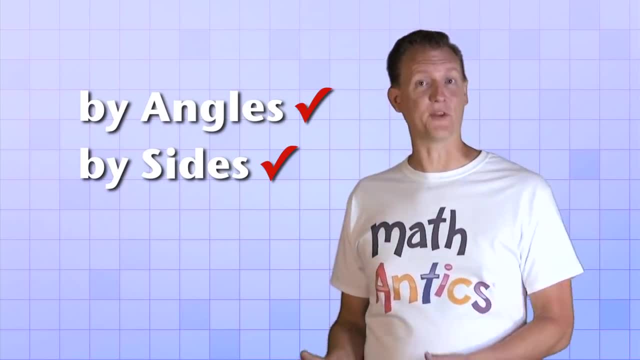 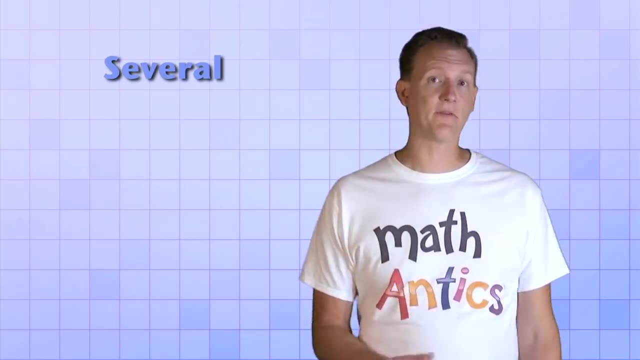 let's see how you can use them together. Yep, you can use them both at the same time. If you classify triangles both by their angles and by their sides, it turns out that there are several possible combinations. To see what I mean, let's list the three classifications by sides. 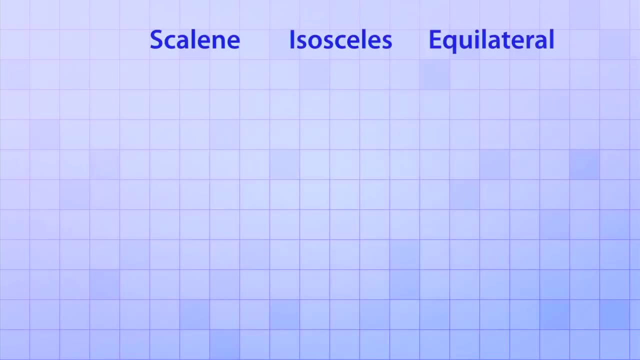 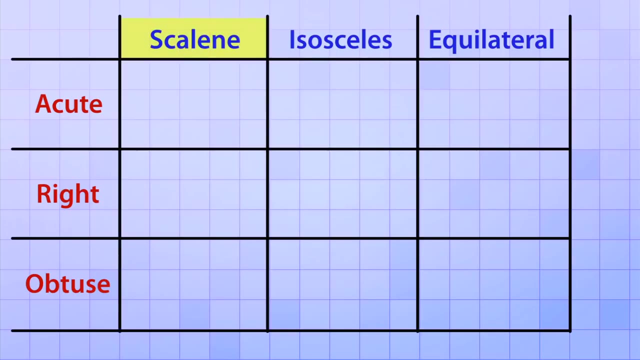 scalene, isosceles and equilateral, and the three classifications by angle: right, acute and obtuse. A scalene triangle can also be a right triangle, like this one, And a scalene triangle can also be either an obtuse or an acute triangle. 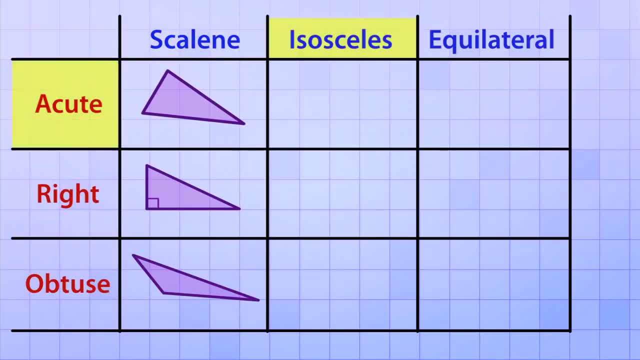 In the same way, an isosceles triangle can also be acute, like this one, or obtuse, like this one, And in one special case, an isosceles triangle can also be a right triangle, like so, But things are different when it comes to an equilateral triangle. 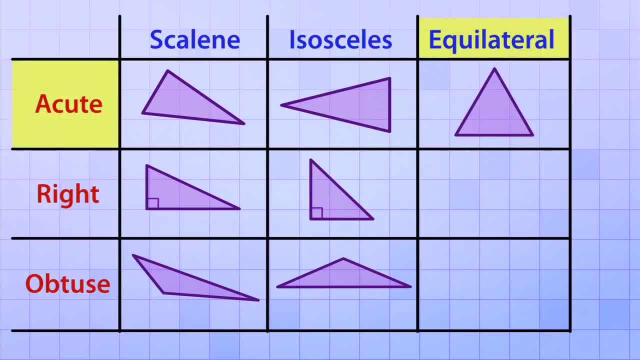 An equilateral triangle is a right triangle. It's always an acute triangle Because all three sides are exactly the same. all three angles must also be exactly the same And since we can't have more than one right angle in a triangle or more than one obtuse angle, all the angles in an equilateral triangle must be acute. 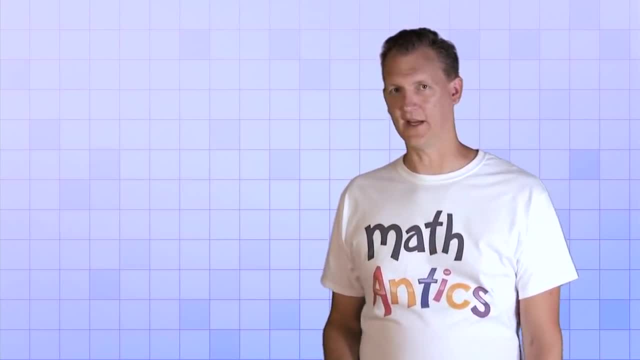 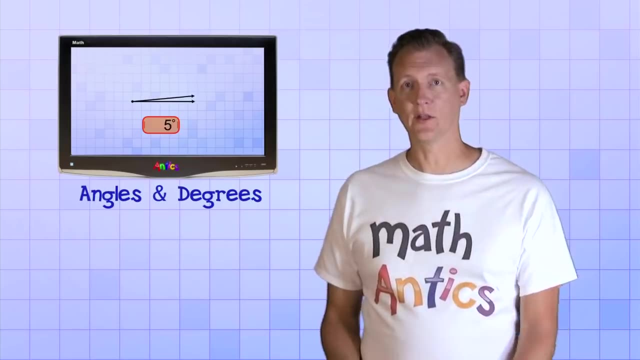 Okay, now that you know all about how triangles are classified, let's learn one more really important thing about triangles. In our video about angles and degrees, we learned that we can measure angles and say how big or how small they are using special units called degrees. 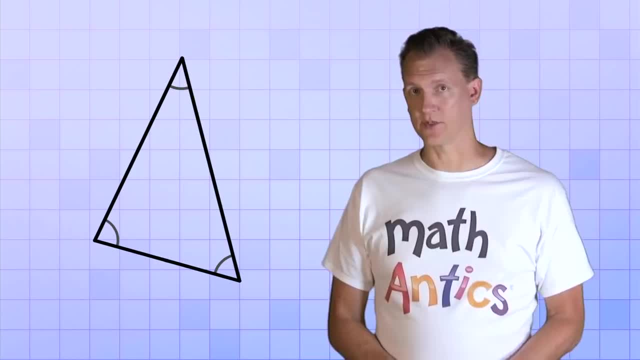 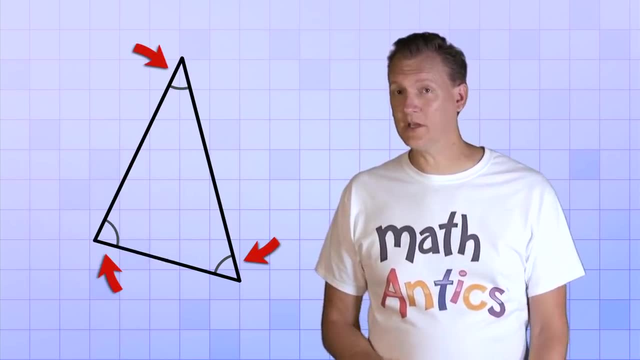 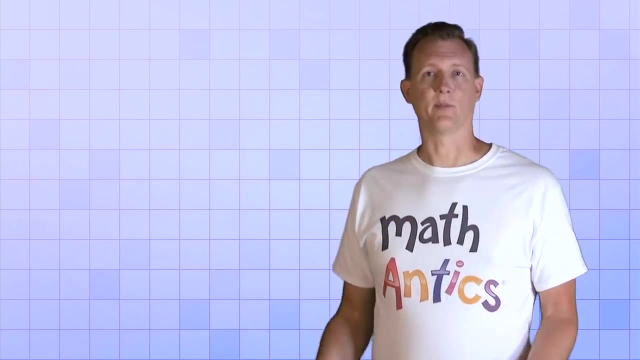 Well, since triangles are always made up of three angles, each of those angles has its own measurement in degrees, And the important thing is that those three angle measurements, if you combine them, they will always add up to 180 degrees, For example. have a look at this triangle. 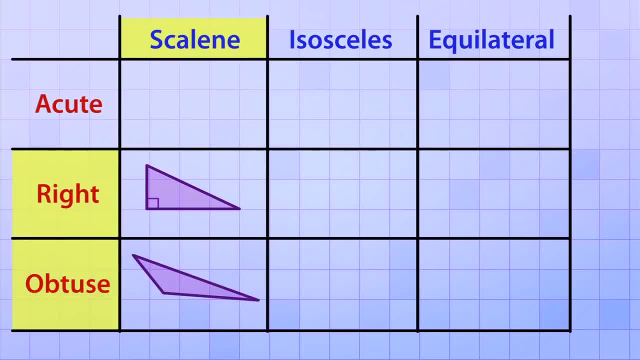 And a scalene triangle can also be either an obtuse or an acute triangle. In the same way, an isosceles triangle can also be acute, like this one, or obtuse, like this one. And in one special case, an isosceles triangle can also be a right triangle, like so. 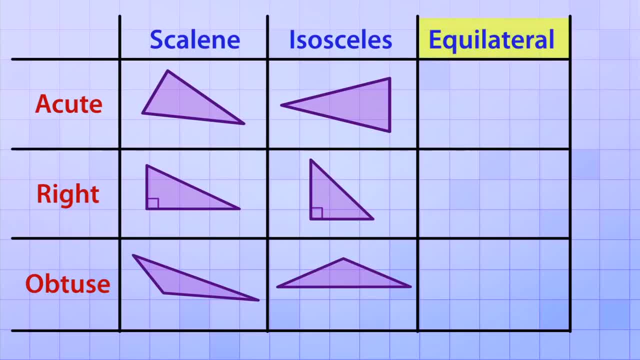 But things are different when it comes to an equilateral triangle. An equilateral triangle is always an acute triangle Because all three sides are exactly the same. all three angles must also be exactly the same And since we can't have more than one right angle in a triangle, or more than one obtuse 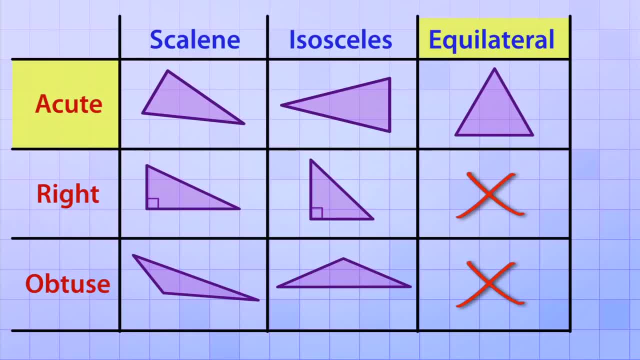 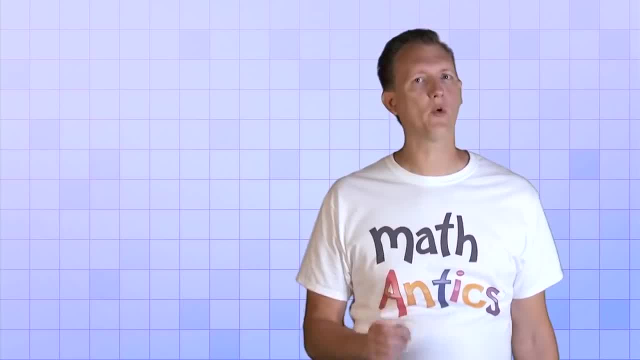 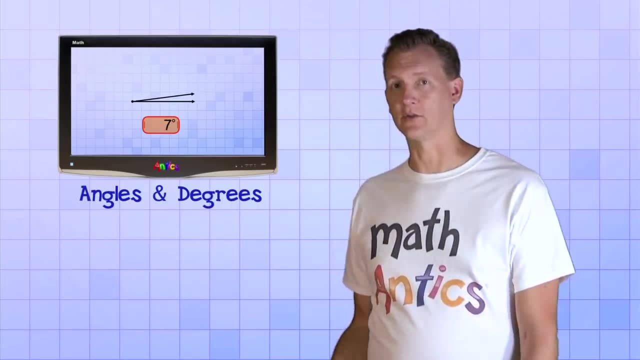 angle. all the angles in an equilateral triangle must be acute. Okay, now that you know all about how triangles are classified, let's learn one more really important thing about triangles. In our video about angles and degrees, we learned that we can measure angles and say: 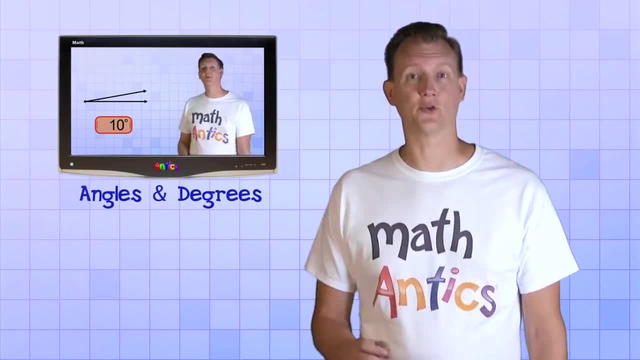 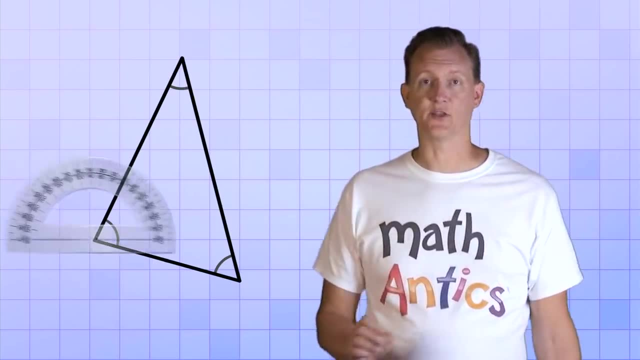 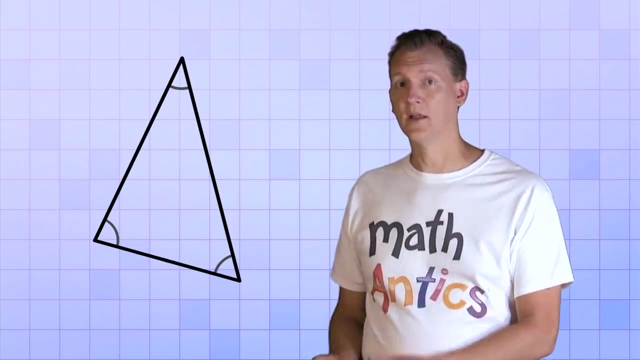 how big or how small they are using special units called degrees. Well, since triangles are always made up of three angles, each of those angles has its own measurement in degrees. And the important thing is that those three angle measurements, if you combine them, they 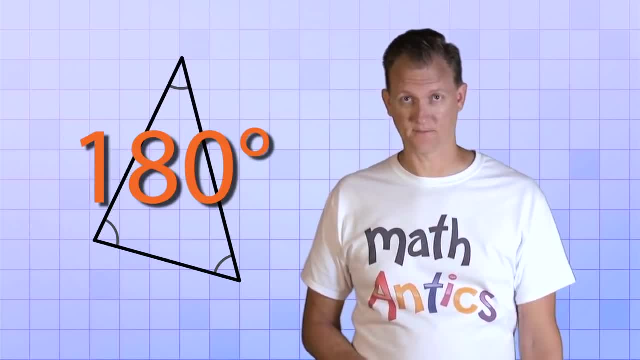 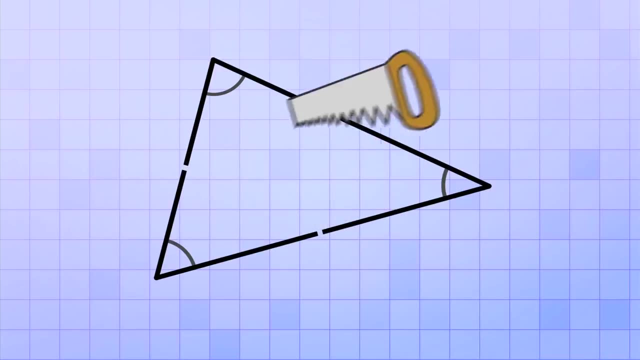 will always add up to 180 degrees. For example, have a look at this triangle. If we were to take a saw and cut it up into three separate angles… and then if we were to take those three angles and rearrange them so that they're right next to each other? 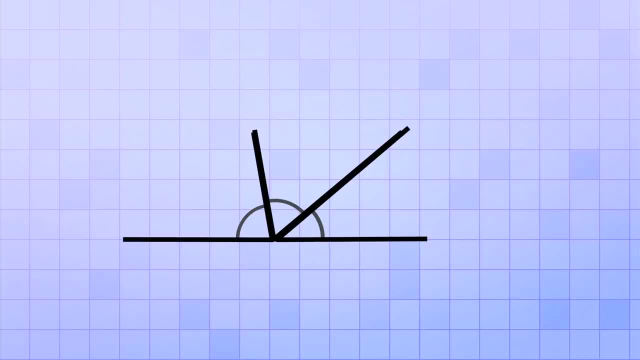 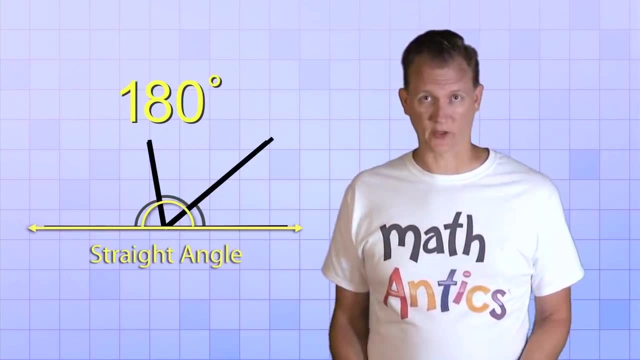 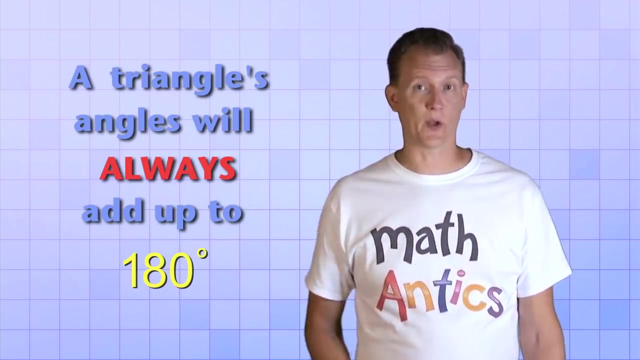 like this. you can see that the total would be the same as a straight angle, That's, 180 degrees, And this will work, no matter what type of triangle it is. Knowing that a triangle's angles will always add up to 180 degrees can really help you. 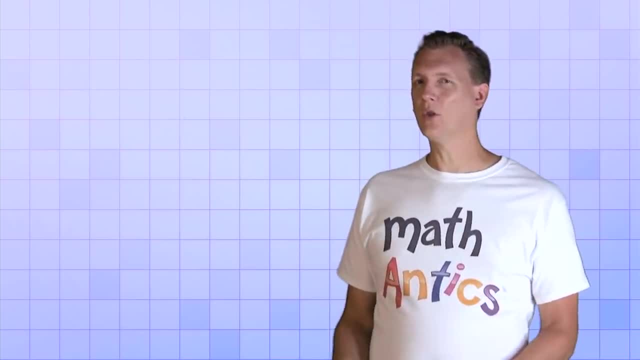 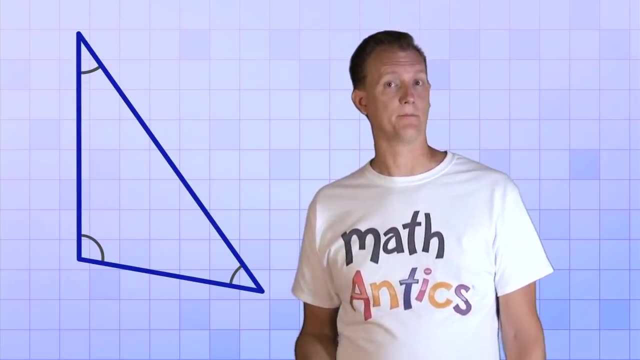 out when solving geometry problems. There's a whole lot of situations where you'll know what two of the angles are, but you need to figure out what the third angle is like. in this problem With this triangle, we're told that one of the angles is 35 degrees and the other is 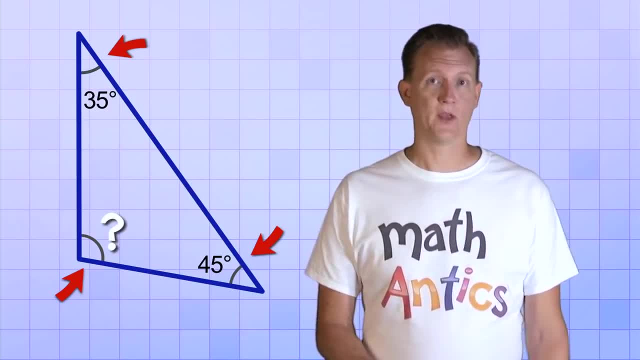 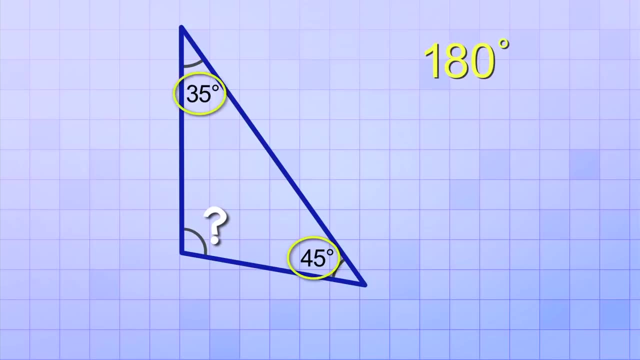 45 degrees, But the third angle is unknown. We need to figure out what it is. Since we know that the total must be 180 degrees, we can just add up the angles that we do know and then we subtract that from 180 degrees to see what's left over. 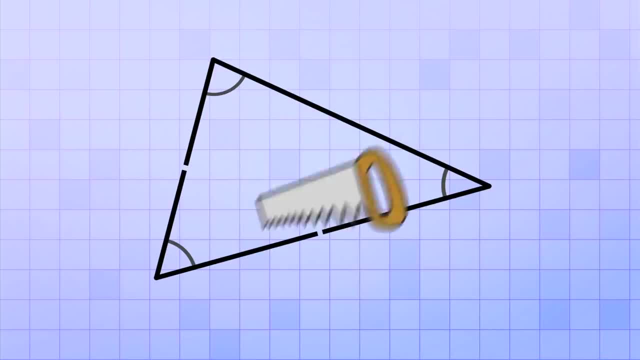 If we were to take a saw and cut it up into three separate angles, and then if we were to take those three angles and rearrange them so that they're right next to each other, like this you can see that the total would be the same as a straight angle. 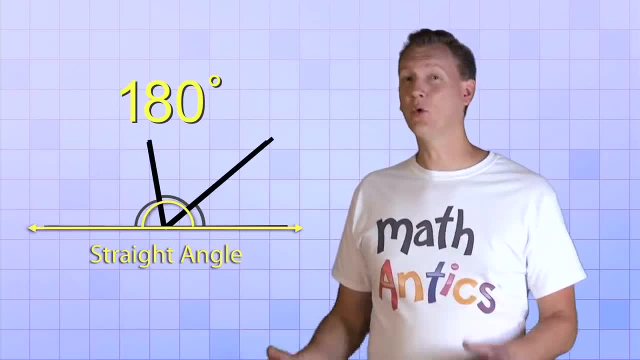 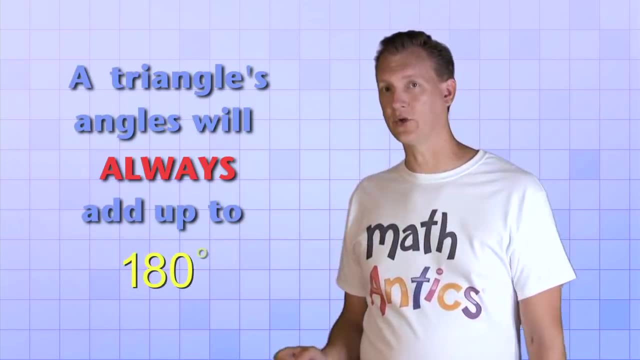 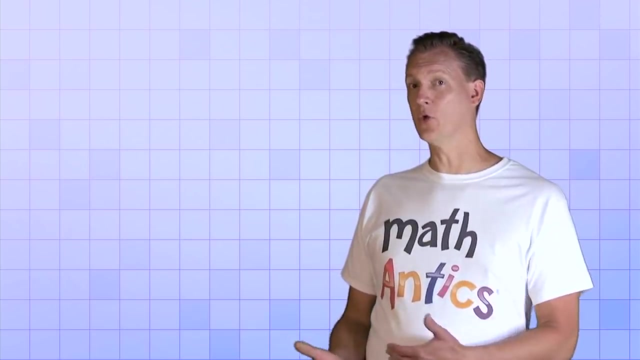 That's 180 degrees, And this will work no matter what type of triangle it is. Knowing that a triangle's angles will always add up to 180 degrees can really help you out when solving geometry problems. There's a whole lot of situations where you'll know what two of the angles 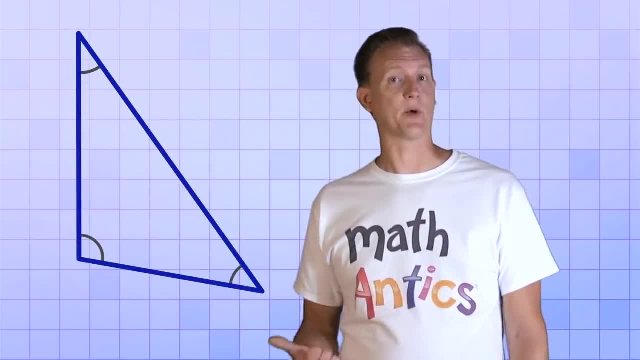 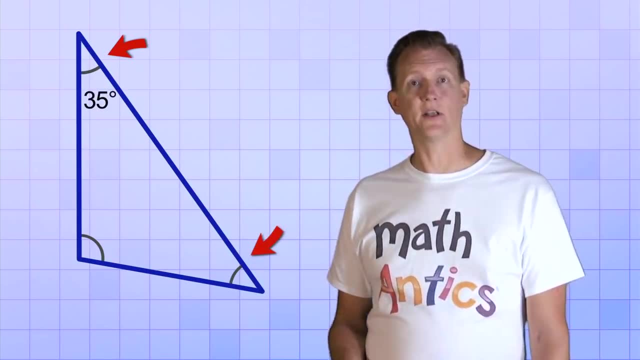 but you need to figure out what the third angle is like in this problem With this triangle. we're told that one of the angles is 35 degrees and the other is 45 degrees, but the third angle is unknown. We need to figure out what it is. 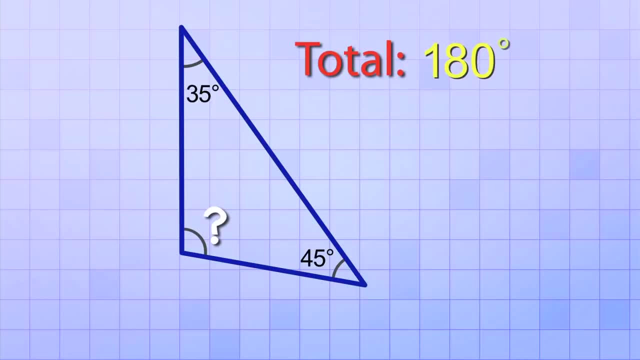 Since we know that the total must be 180 degrees, we can just add up the angles that we do know and then we subtract that from 180 degrees to see what's left over. The leftover amount must be 80 degrees. the amount must be the measurement of the unknown angle. 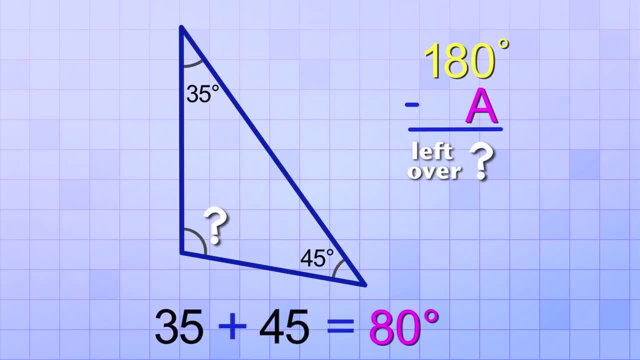 So 35 plus 45 equals 80 degrees, And when we take that 80 and subtract it from 180, we get 100 degrees left over. That means that our unknown angle is 100 degrees, And you can always check your answer by adding up all the angles to make sure you get 180. 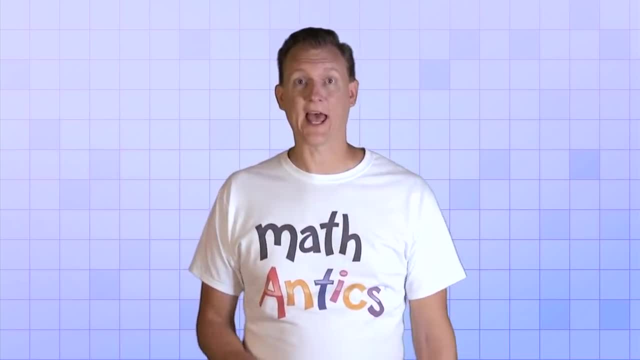 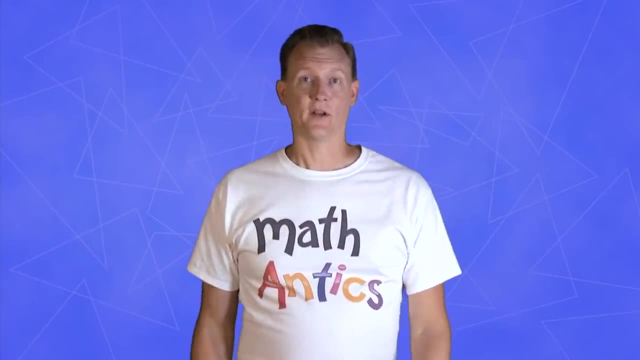 So you can see why it's so important to know that a triangle's angles add up to 180 degrees. Well, that's all we're going to learn about triangles in this video. Remember, the key to really learning math is to do it. 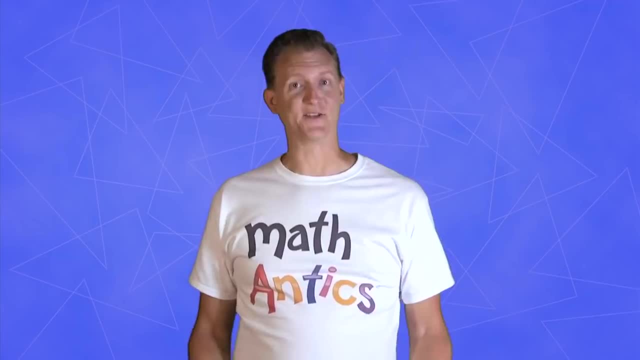 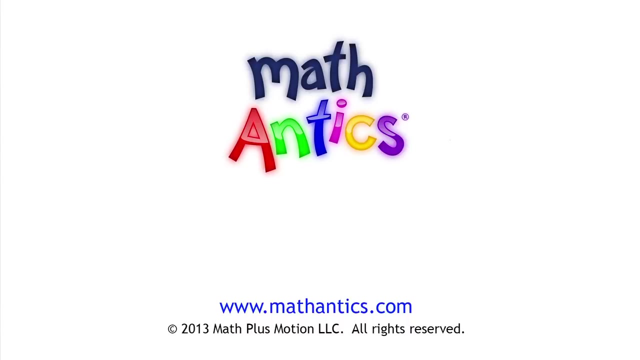 So be sure to practice by doing the exercises for this section. As always, thanks for watching Math Antics and I'll see you next time. Learn more at wwwmathanticscom.